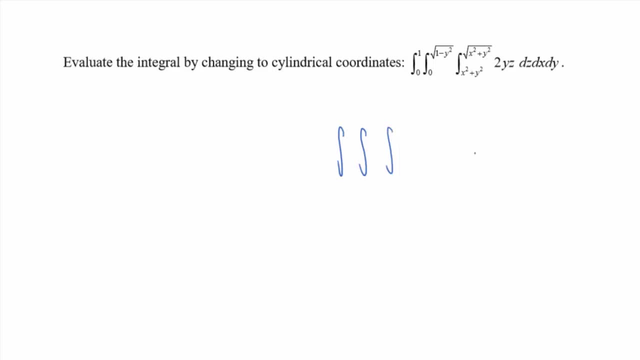 so you get the right extra factor in there. So what's the correct volume element You need an extra factor of? I might need some extra room too. So r dz dr d theta. Usually you can pretty much count on the order being dz dr d theta. It doesn't have to be, It's just. 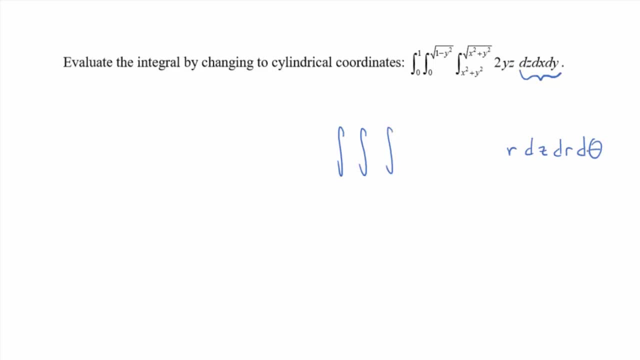 why not stick with one? because one's not easier than the other? Not usually, anyway. Okay, and then we might as well handle the integrand while we're here, What's y in cylindrical coordinates? Same as polar? Okay, I'm going to write the 2 out here. 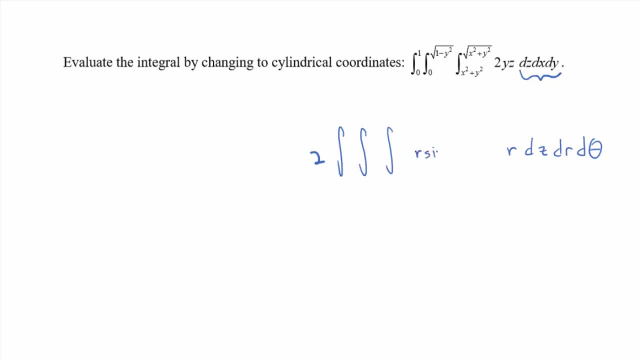 and then r sine theta, And then what's z? Trick question. It's z right In cylindrical anyway. Okay, now this is where the stuff that we're going to do is going to be. from the very first chapter, And I don't know if you remember, but I warned you. These are the 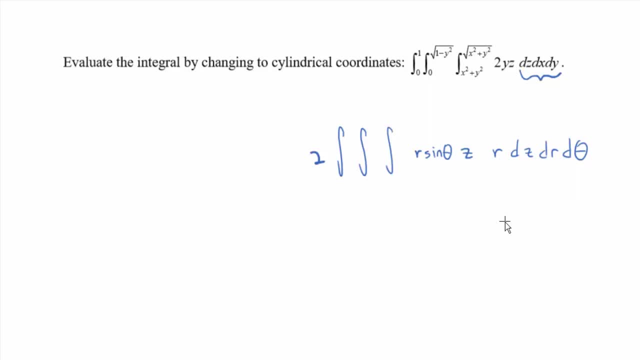 surfaces we learn calculus on. That's what I meant when I said you got to learn how to graph this stuff. So this bottom limit here. do you remember what that graphs to be? A parabola right? A circular parabola actually. So you think of it as z. This is the bottom limit on the z right. 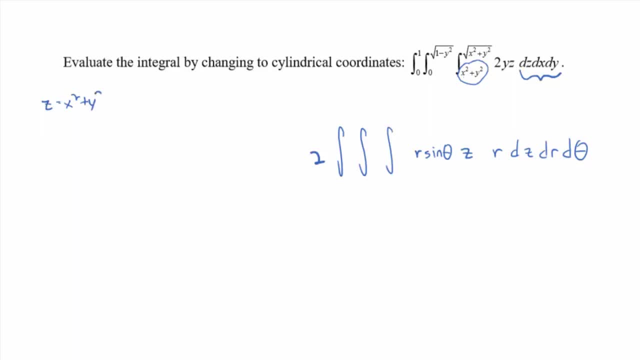 So z equals x squared Plus y squared. I think we could actually get away without graphing it here, but you should have in your mind a picture of what it looks like. So it looks like that satellite dish, kind of elongated satellite dish. None of them go this deep right, But at least not proportionally. That's the best. 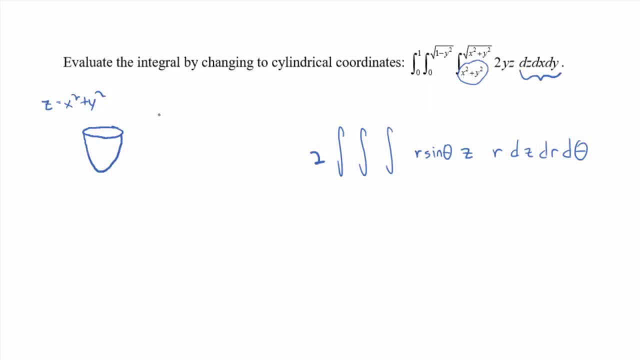 I can do today, apparently, And then. so that's kind of the floor right. And then, what's the ceiling? What's the ceiling going to be? Okay, set z equal to this. It's a surface in space. What is it? 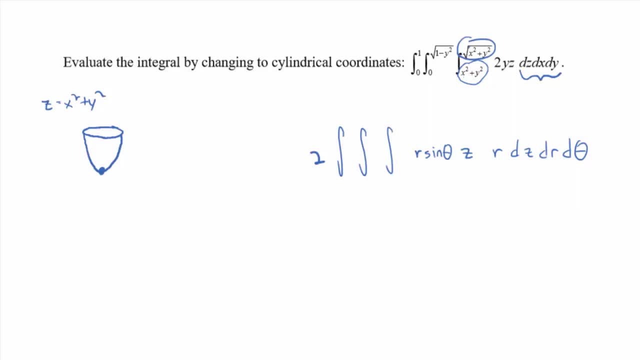 No, It's a cone- Top half of a cone for crying out loud, right, And I'm just kidding, It's hard to know all this stuff, right? But you got to get comfortable with it to be good at this stuff. 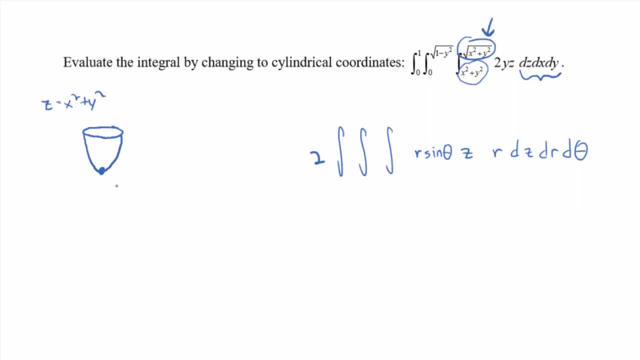 Now, interestingly, the vertex of this cone is the same in the same spot as the vertex of the paraboloid right, But it's kind of skinnier, at least for part of the way, And it'll look something like that on the inside. And you know, when they intersect they're going to have the 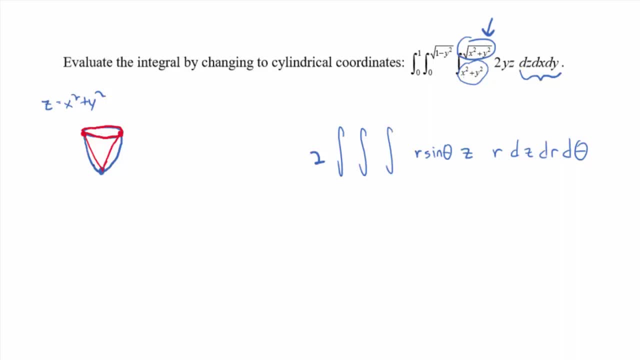 same curve of intersection up at a height of z equals one, I suppose. right, So you can then think of the cone as the ceiling And then you know when you have the cone as the ceiling. you can think of the cone as the ceiling And then you know when you have the cone as the ceiling you. 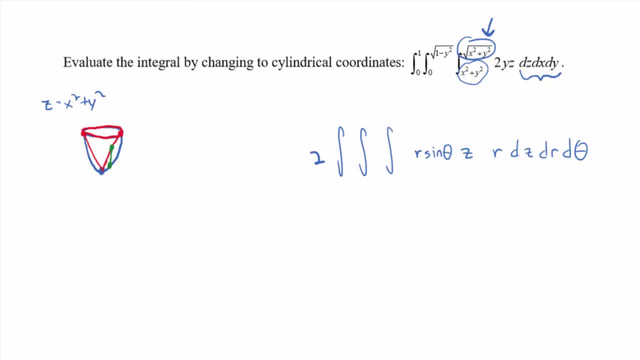 and the paraboloid is the floor. That's how it makes sense visually. Anyway, for this particular one, I think you'd get away without drawing that picture, because it's a direct transformation to cylindrical coordinates. What is x squared plus y squared in cylindrical? 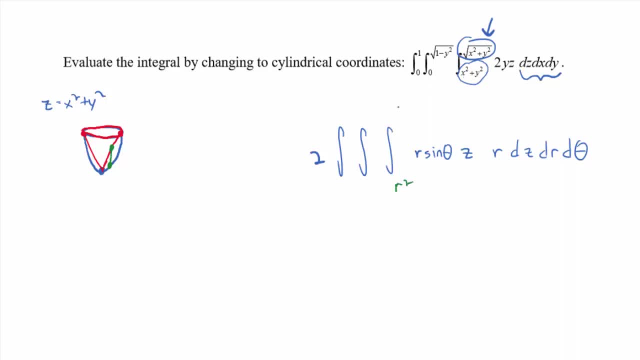 R squared, and then the square root of r squared would be the top right, which would just be r- the ceiling. Does that make sense? Okay, And then, as far as the outer limits of integration go, well, it might not be the full circle of intersection. 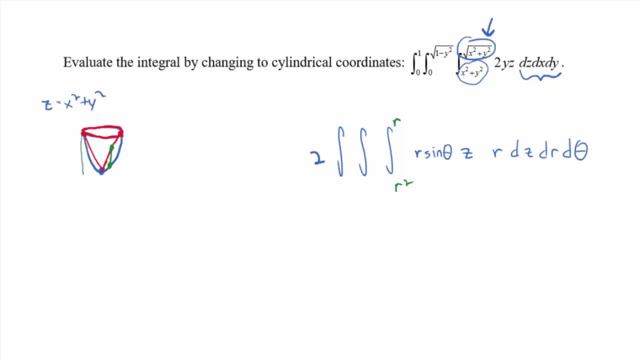 as the boundary right. But when you project down without the zeros there, if it went the full way, you'd get this circle of intersection, wouldn't you? Again, more stuff. you don't necessarily need to get the right answer here, but it does help, I think. 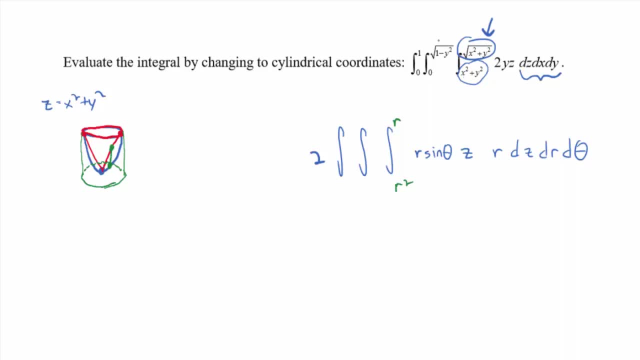 What does? okay, zero. I think it's clear what zero is. but what does this guy describe? Okay, it's the limits on x, right? The middle limits of integration are the limits on x. so x goes from zero to root one minus y, squared right. 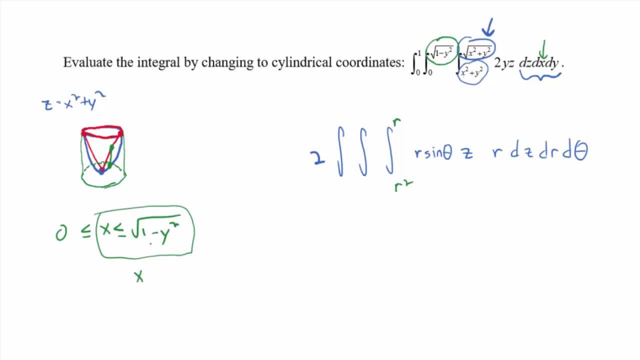 If you take this boundary equation given by the upper limit on x, symbolically, you can recognize that as part of a circle by just squaring both sides and putting it in standard form: If you square both sides you get x squared equals one minus y squared and add y squared to both sides. 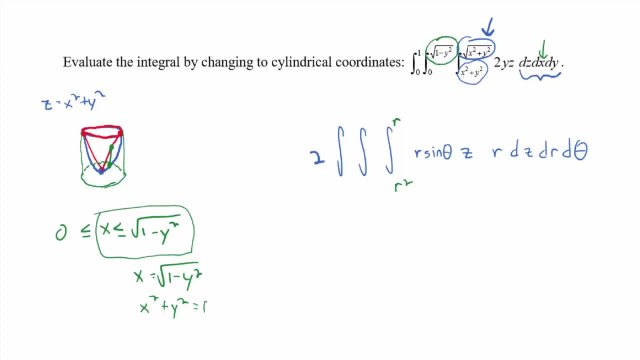 you get x squared plus y squared equals one, don't you? So that, okay. so that's a circle of radius one, But I don't think we're talking about the whole circle here, are we? Okay? So imagine projecting this guy. 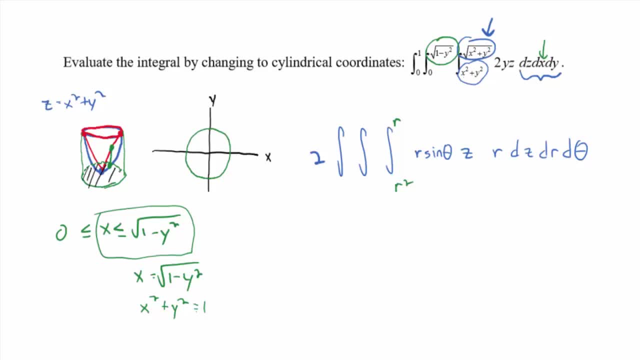 you get the circle as the boundary and the interior as a disk, right, But the outer limits of integration limit how much of the disk we're going to integrate over. And if you look at the original integrand it's actually set up the outer differentials dx dy. 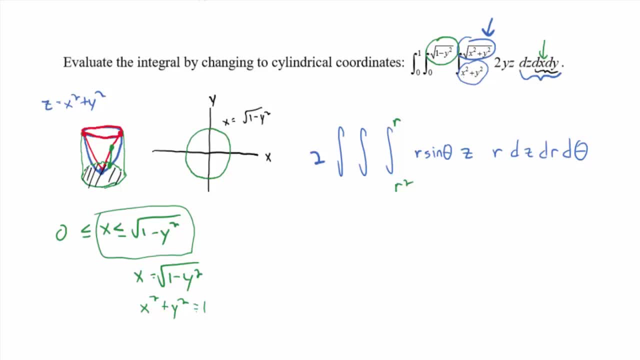 which corresponds to what kind of rectangles? Horizontal, But the horizontal rectangle only goes from zero- x equals zero- to the circle. So visually going backwards, that's if you were setting up the integral in the first place, that's what the picture would have looked like. 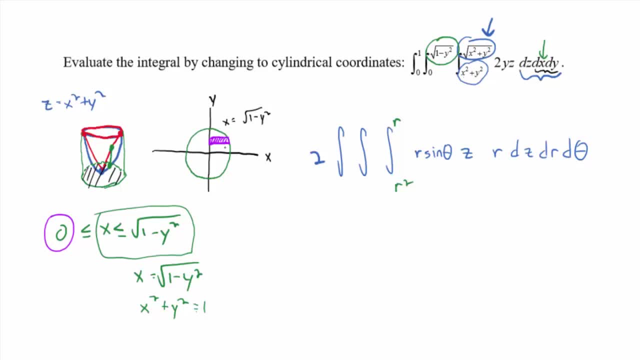 So what part of the circle does x equal the square root of one minus y squared describe? Not the top part, not the bottom part. Well, really, if you're just talking, x equals square root of one minus y squared, it's really the right-hand part of the circle, right? 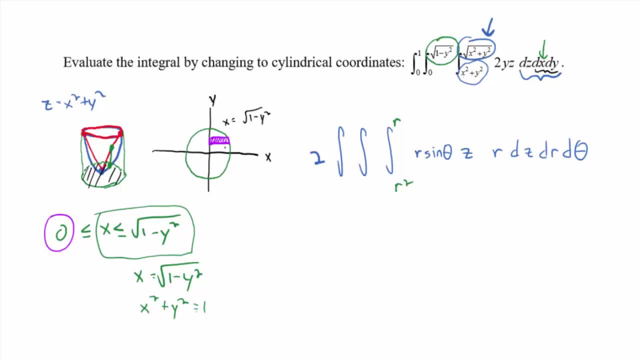 Now we are going to be limiting it to the first quadrant because of something else, But just talking about that equation, x equals the square root of one minus y. squared is the right half of the circle, right. However, knowing the outer limits- the original outer limits- y goes from zero to one. 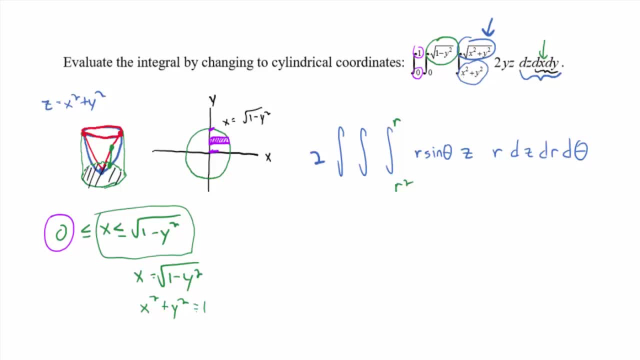 Oh, that's down here to here, right? So that does put you in the first quadrant, doesn't it? So it's the outer limits that give you that you're limited to the quarter disk, really, Okay. so now that we know what we're integrating over in a type of cylindrical 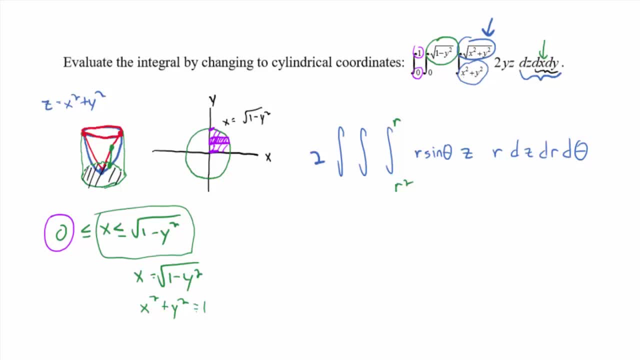 well, really, it's polar right for the outer limits of integration. what does r range from? Think radially from the origin. Think drawn a spoke. What does r range from Zero to one? That's a circle of radius, one right.